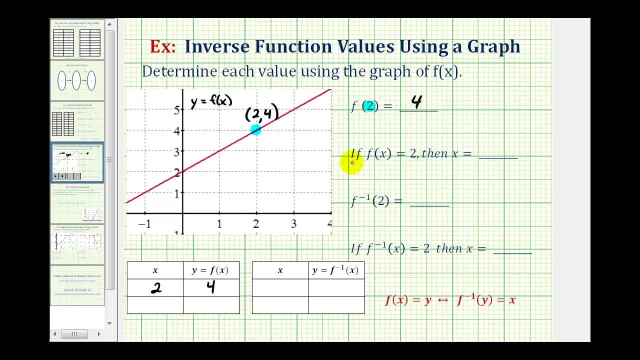 is four. Next, we're told: if f of x equals two, determine the value of x. Well, here, two is the output or the y value of the function. So, going back over to our graph now, we want to find where the y coordinate equals two. 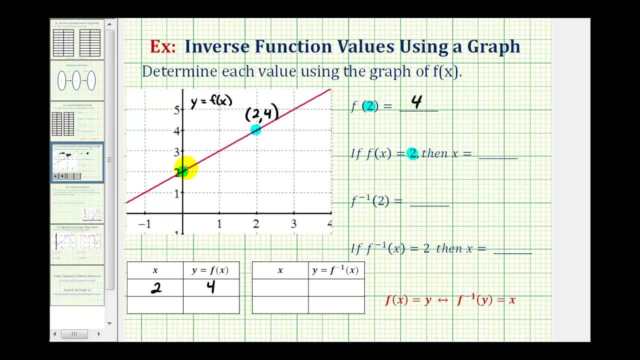 Well, the y coordinate is equal to two. right here on the y axis, The coordinates of this point would be zero, two. So when the function value or y value is positive two, the x value or input is equal to zero. So if f of x equals two, then x equals zero. 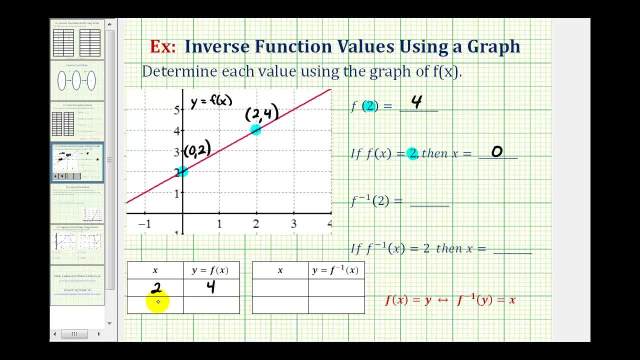 Again, if we want to record this information in a table of values, we would have: x equals zero and y, or the function value is equal to positive two. Now, the reason I wanted to record this information in a table is because if we complete a table of values for the inverse function, 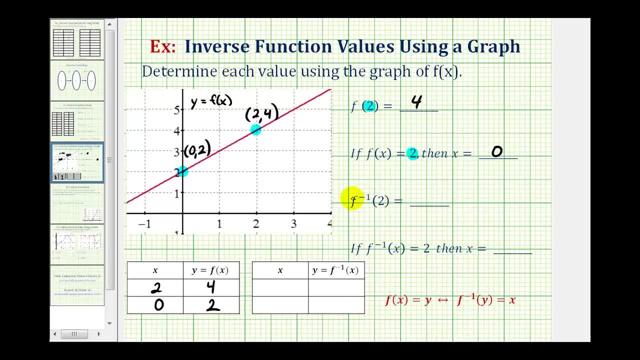 it'll help us answer these last two questions involving the inverse of function f. Remember f and f inverse undo each other. So if the input for function f is two and the output is four, then if the input for the inverse function is four, 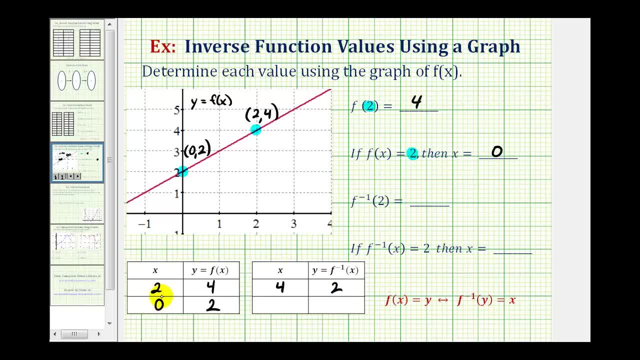 then the output would be equal to two. If the input for f is zero and the output is two, then if the input is two for the inverse function the output would be zero. So we can see these two functions are undoing each other. 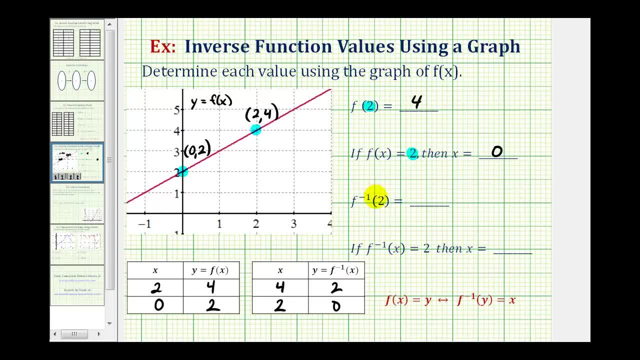 So looking at these last two to evaluate f inverse of two, we need to recognize that this two here is the input into the inverse function and we want to determine the output or function value. So, looking at this table of values for the inverse function, 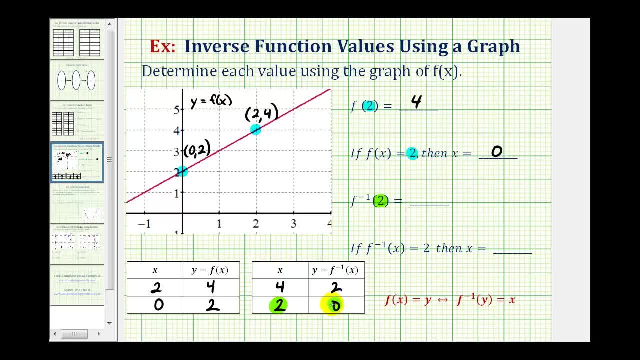 notice: when the input is two, or x equals two, the output is zero. So f inverse of two is equal to zero. If we wanted to find this value using the graph, we'd have to recognize that for the inverse function, this y coordinate or function value would be the input. 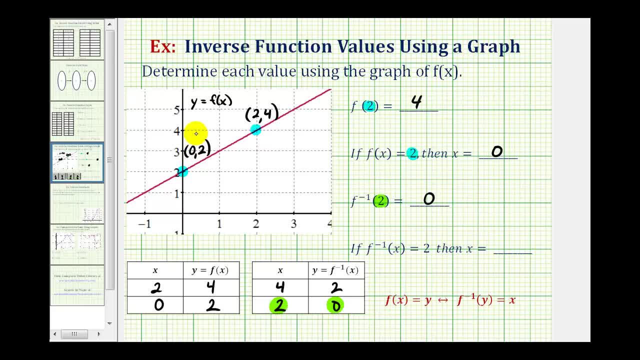 and the x coordinate, or zero, would actually be the output. And that can be a little tricky at first, and that's why it's often helpful to record the information about the inverse function in a different table. Looking at the last question, if f inverse of x equals two, 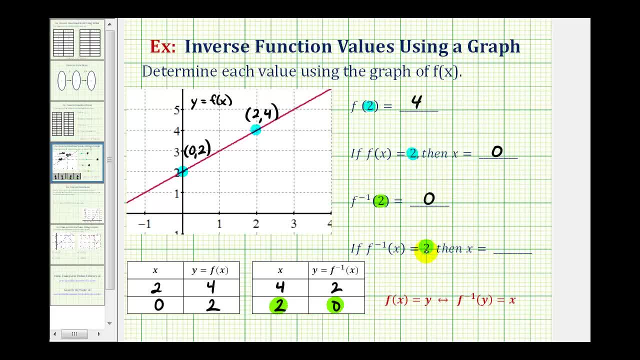 meaning if the output of the inverse function is equal to positive two, we want to determine the x value. So, again, looking at our table of values for the inverse function, notice if the output for the inverse function is two, the input or x value is equal to positive four. 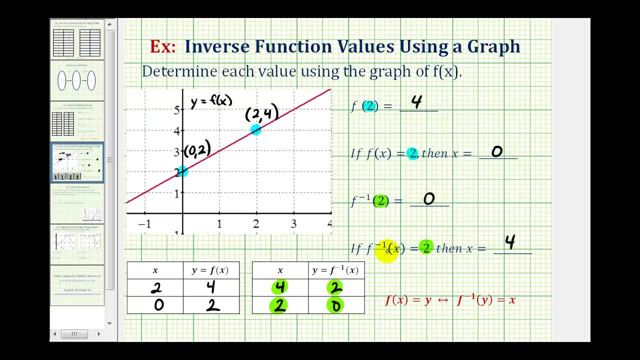 Again, looking back at the graph, we'd have to recognize that if f inverse of x equals two, this two here would be the output of the inverse function and the input would equal this four. here There is one more important connection I'd like to make. 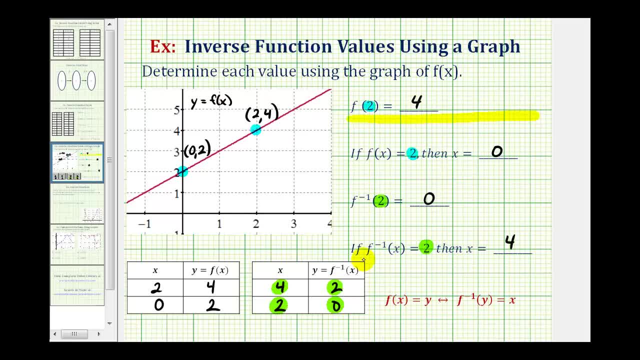 If we take a look at this first question and this last question, there is a connection. Notice. when the input into the function f is two, the output is four, and if the output of the inverse function is two, then the input is equal to four. 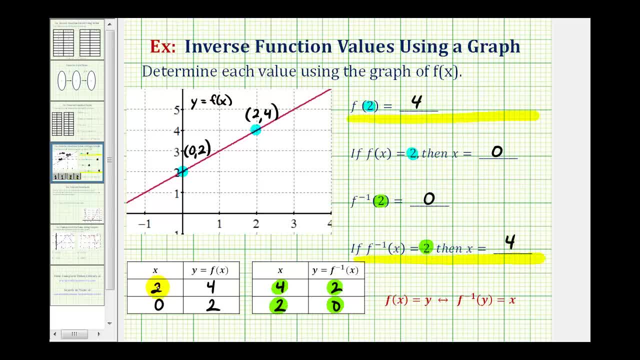 This information here is the same information we have here for this first row of these two tables, And then this question here and this question here are also related. For function f, if the output is two, the input is zero, And for the inverse function, if the input is two. 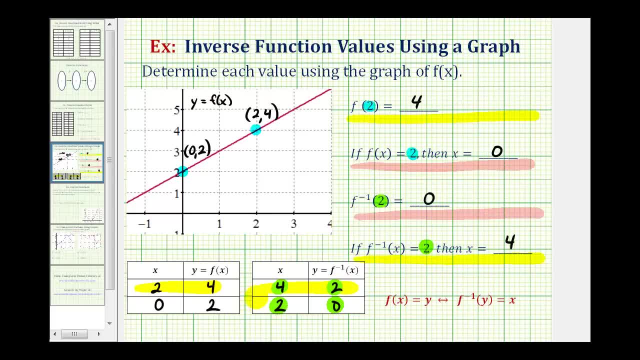 the output is zero. These two questions here emphasize the relationship between the function f from these two rows here. I hope you found this helpful. Thank you. 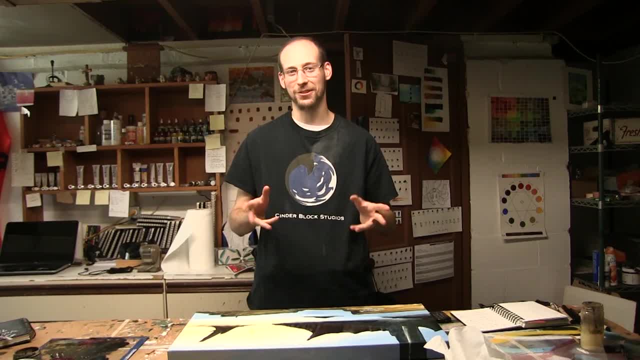 Hey everybody, Ben here from Cinderblock Studios, and I'm back with another video about color theory. This particular video is probably a little weirder because it's both art and it's science. so let's get sciency, That's a bit more like it. so today let's talk about